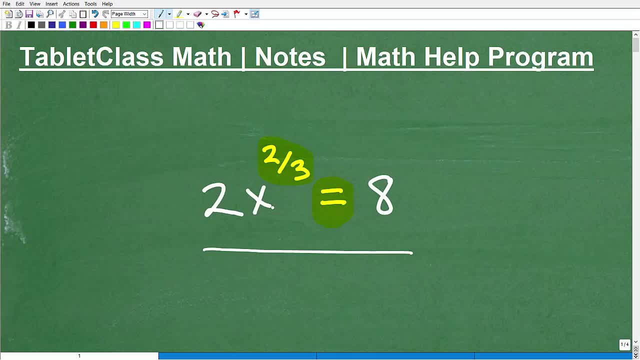 equations that involve rational exponents, you don't need a calculator. Matter of fact, you know the problem like this could be given to you on a quiz or a test where your teacher says no calculators allowed. So we're going to cover. 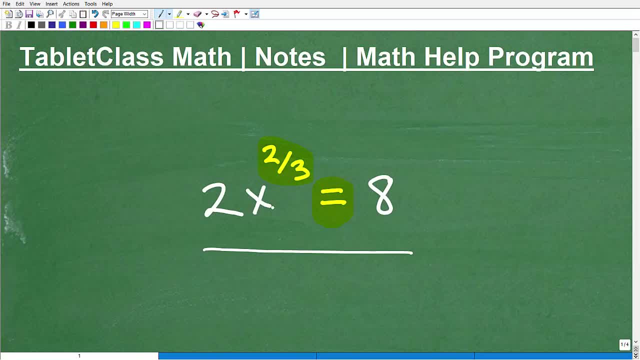 how to solve this particular problem, And it'd be a good overview to this topic of solving equations with rational exponents. And we're going to get to this in just one second. But first let me quickly introduce myself. My name is John. I'm the founder of tablet class math. I'm also a middle and high 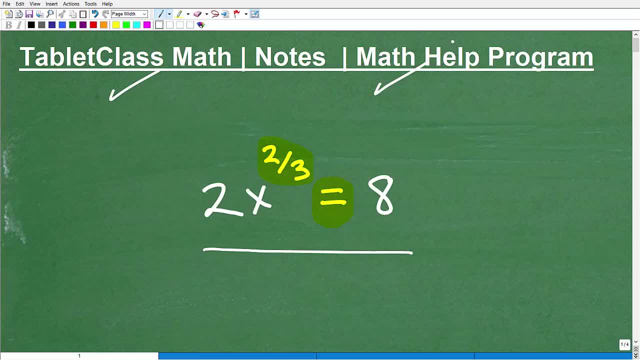 school math teacher and over several years I've constructed what I like to believe is one of the best online math programs there is. Of course, I'll let you be the judge of that statement, But basically I have 100 plus different math courses, So I have all the main courses like pre-algebra. 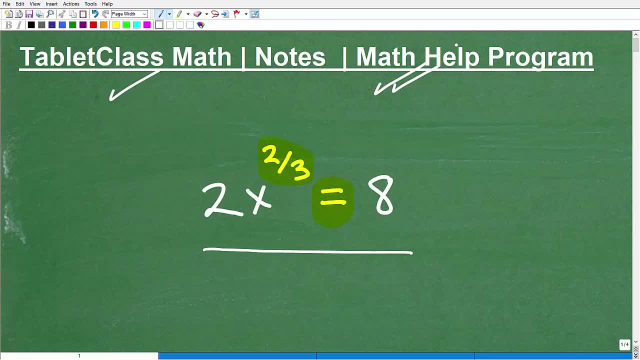 algebra one: geometry. algebra two, algebra three, algebra four, algebra five, algebra six, algebra seven and algebra eight and algebra nine. I'm going to be launching my pre calculus course here, But I have several, many, many test preparation math courses. So for those who are studying for, 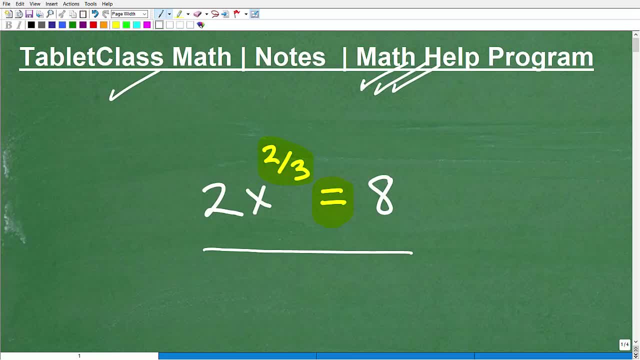 the GED, SAT, ACT, GRE, GMAT, Alec's, ACCA- There's a ton of different reasons- or teacher certification, nursing entrance exam. There's a lot of huge, very, very important critical exams that people take. They have to pass, and there's a 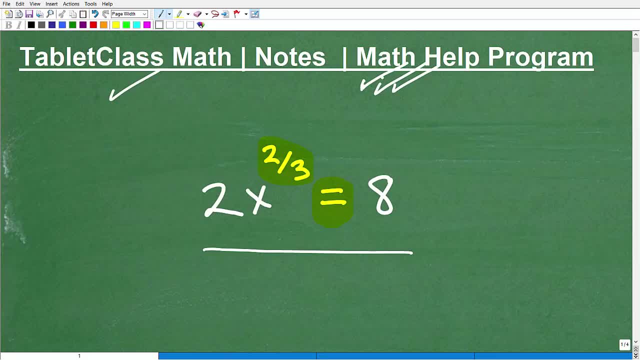 math component to them. so I recognize that I've developed over the years very comprehensive math test preparation courses. so if you're studying for a particular exam, check on my full catalog. I likely have your course and if I don't, drop me a line in our contact form and I'll get back to you. I also work a lot. 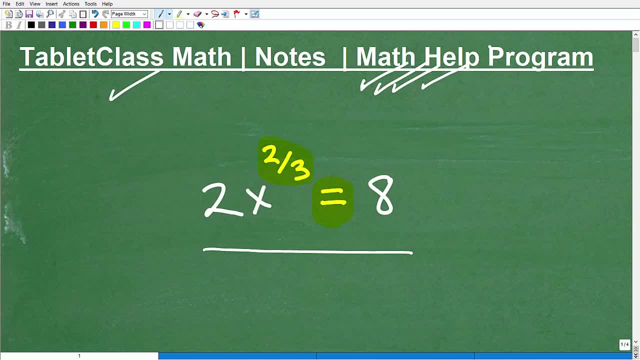 with independent learners. so if you're like a homeschooler, for example, I have a great homeschool learning system- and then, obviously, if you're just struggling in your current math course- let's say you're taking algebra one, algebra two and you need additional help- I could help you out now, one thing you could do: 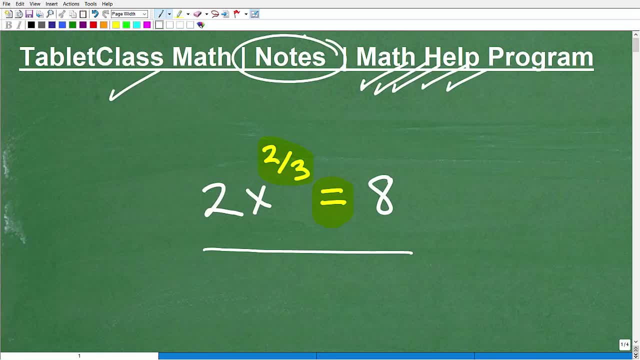 to help yourself out is to take fantastic math notes. that is absolutely just the foundation of learning math and kind of over decades of teaching math, it's just that my golden rule is: those students who take great math notes almost always get great math grades, and the reverse is true. those students are 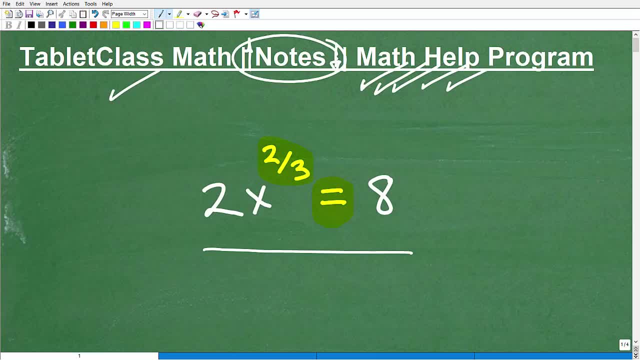 just like. nah, I don't like to take notes, you know, I'd rather do my homework or look at my cell phone or talk to my best friend. listen, I get it. I'm not trying to make you feel bad. I'm not trying to make you feel bad. 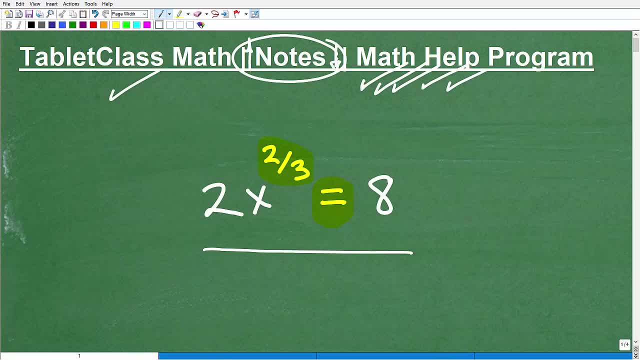 but let's be honest, right, there's a huge amount of distraction, and it's going on when you're learning in class. okay, and the one way to avoid all those distractions is what to be engaged. you can stay focused on an activity that will keep you focused. all right, and that is note-taking if the teacher is. 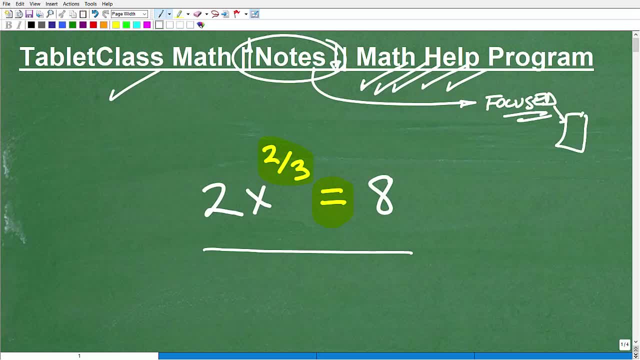 constantly teaching. you have to be, you know, concentrating to put this in to your notes, and your notes should be fantastic, all right, you should be able to read them. you don't want to just be like scribble scratching like this, like I used to be back in the good old days- yeah, so I know, I used to be slot. 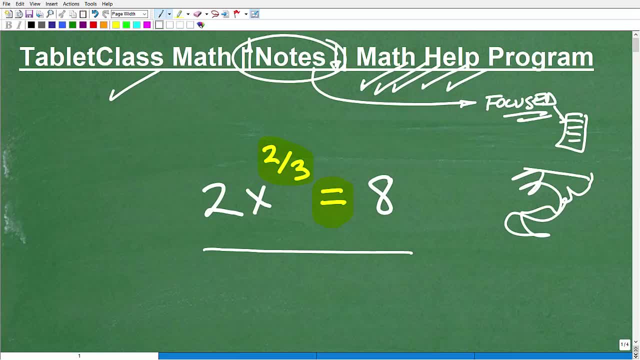 very sloppy and, matter of fact, I would take all these notes and I'd be like, oh, look at me. and then I'd look and like, what did I write down? I don't even understand my own notes. so, if that's, you listen. a lot of people are like that. 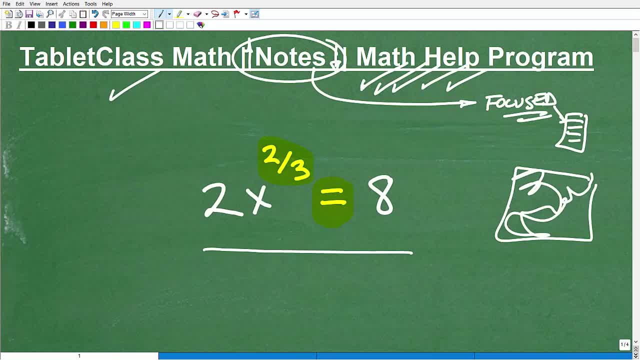 that's why note-taking is a discipline, it's a skill, and they really got to stay focused. now, as you're improving in your note-taking- and hopefully you know this will motivate you to do so- you still need something to study from, so I offered detailed, comprehensive math notes to include pre-algebra. algebra one: 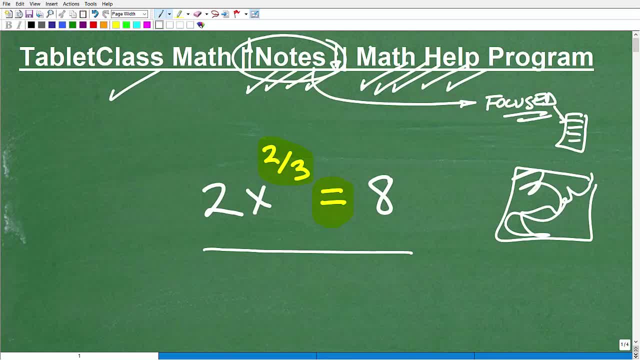 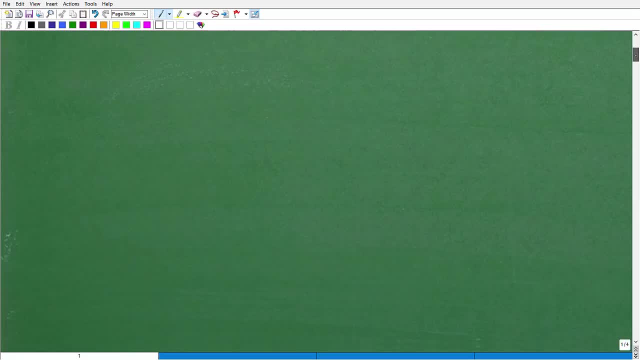 geometry, algebra two and trigonometry. okay, so let's get into how to solve this particular equation involving rational exponents, and I'll show you how to do this without the aid of a calculator. of course you could use a calculator here, but we're doing, we're going to go ahead and just show you the best approach, how. 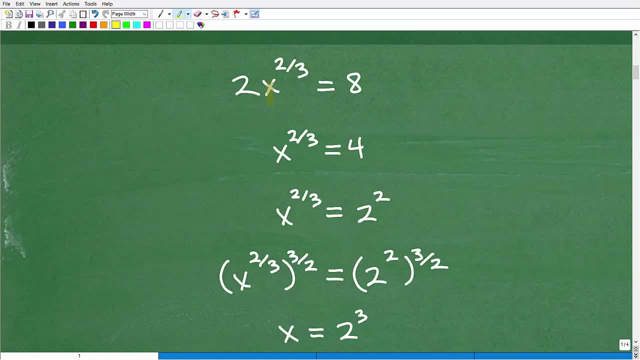 to do it now. the first thing you need to do when you're solving an equation involving rational exponents is to solve, for the rational exponent and the variable component, this part of the problem. you want to get this by itself and you can see we have this by itself. so how do I do? 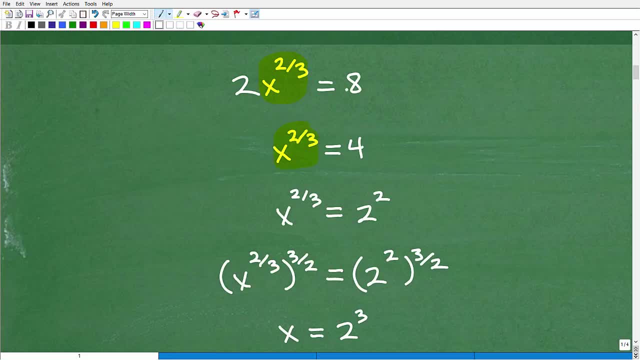 that. well, you can kind of see, this is 2 times this equals to 8. so if I had 2x is equal to 8, how would I solve for X? well, yeah, I would just simply divide both sides of the equation by 2. I get X is equal to 4. so same thing here I'm going. 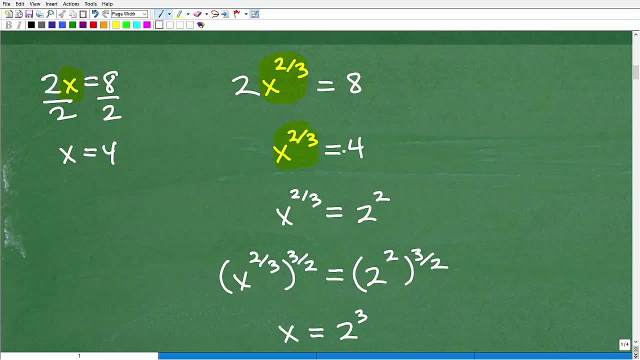 to divide both sides of the equation by 2 and I get X to 2. thirds is equal to 4, so this is where you want to really have the problem set up now. anytime you're dealing with equations that involve powers and exponents and you have a number on one side of the equation, what's nice and 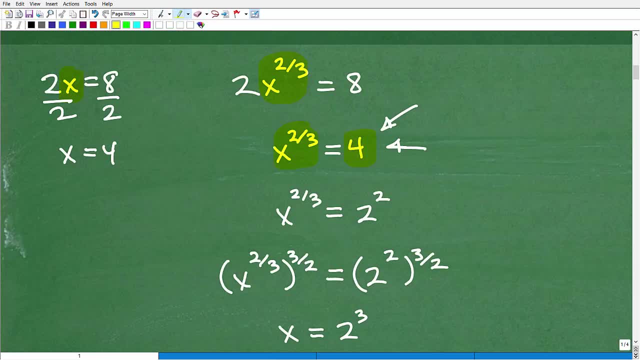 simple this way: think in terms of how can I express this number on this one side of the equation, as a power in and of itself. so here I have the number 4. you're like, oh okay, well, 4, isn't that equal to 2 times 2? in fact, it is so. 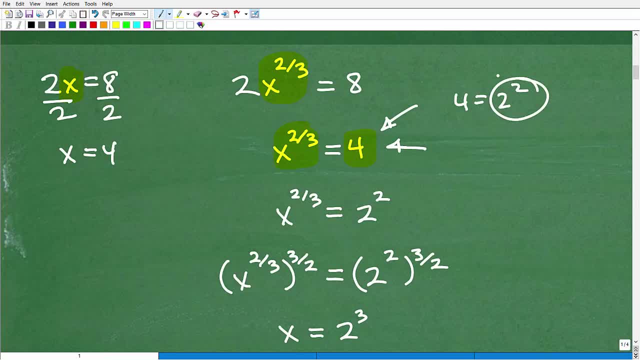 let's express 4 in terms of a power. so when you're dealing with powers and exponents, So try to get. oftentimes, especially if you're not allowed to use a calculator on this quiz or test, that's almost a dead giveaway. 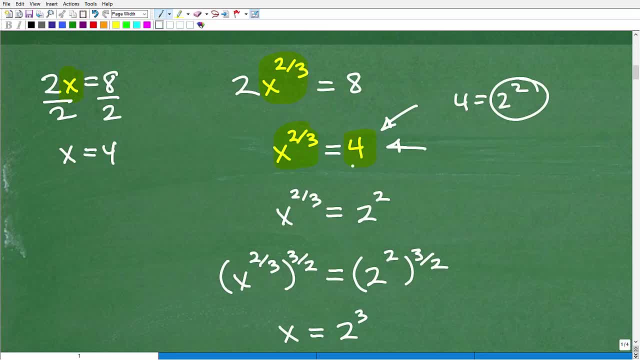 You're going to have to take this number and express this as a power. So 4 is the same thing as 2 squared. So now I have my problem kind of all set up to solve. So I have x to the 2. third power is equal to 2 squared. 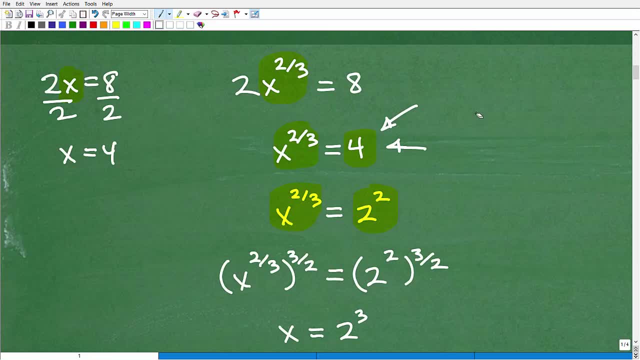 Now one thing that you need to know. okay, about these expressions, let's just do a quick review here: x to the 2 thirds. okay, this is the same thing as this. all right, This expression, x squared. this is the cube root of the expression, the cube root of the square root of x squared, right. 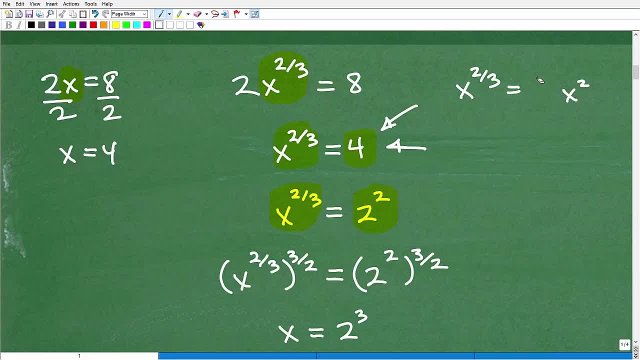 The cube root of x squared. excuse me, that's the way you say that. Now I don't want to go, let me write that a little bit better. Okay, that's what this is equal to. So you're going to have to be able to rewrite radicals into rational exponents. 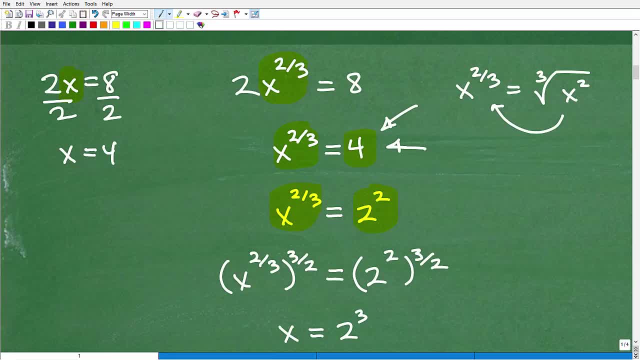 And that's kind of a different topic, but you need to be aware of that. So some of you can be like: well, isn't this equal to this? In fact, it is okay, But what we're going to do is solve this equation sticking with rational exponents. 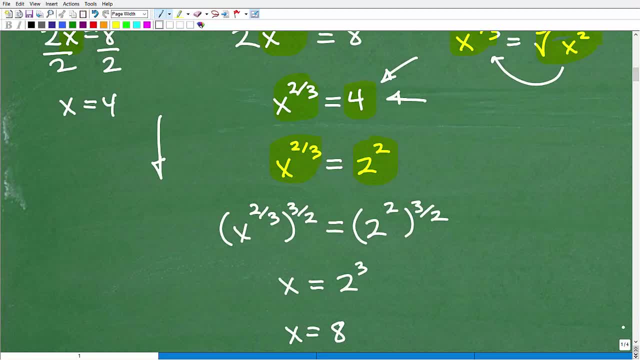 We're not going to rewrite this in terms of radicals. We just need to know that those are equivalent. Okay, so I want to solve. I want to solve for x, but I have x to the two-thirds. all right, I want to solve for x, so I want x by itself, right. 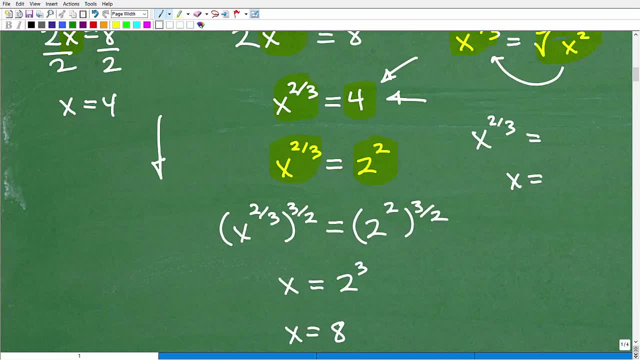 X, like this, x. I don't want x to the two-thirds, but x to this. you know when I'm solving for x, this is really x to the first power. okay, We, you know we write it as x, but it's really x to the first. 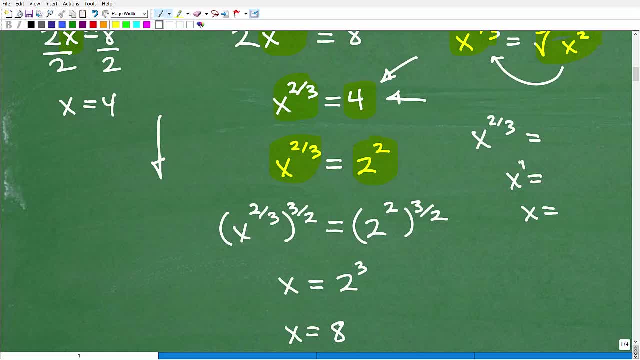 So I'm saying: well, how can I make an x to the two-thirds into a one? Well, that's pretty easy. okay, I can take this two-thirds and raise that to the three-halves power, because when I distribute three-halves to two-thirds, okay. 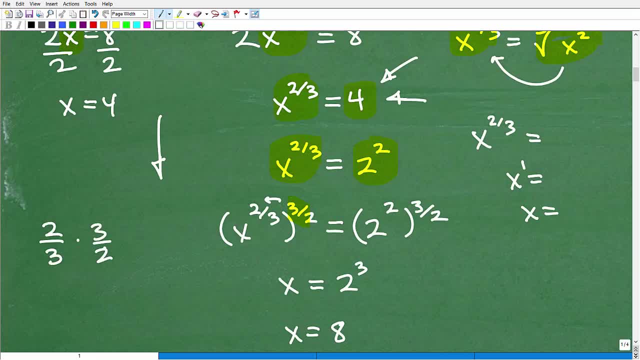 Two-thirds times three-halves And if you're not familiar with how to take a power to a power, check out some of my other videos in my algebra playlist. But this is going to be obviously all this cross cancels. 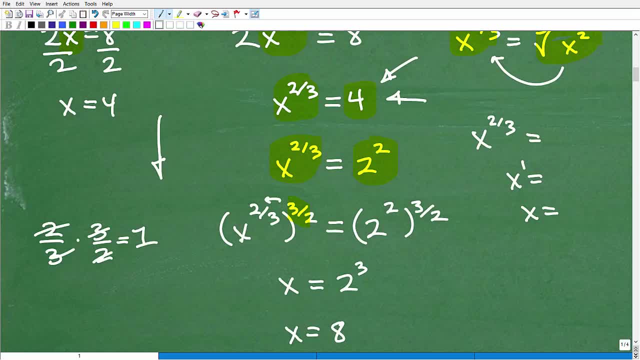 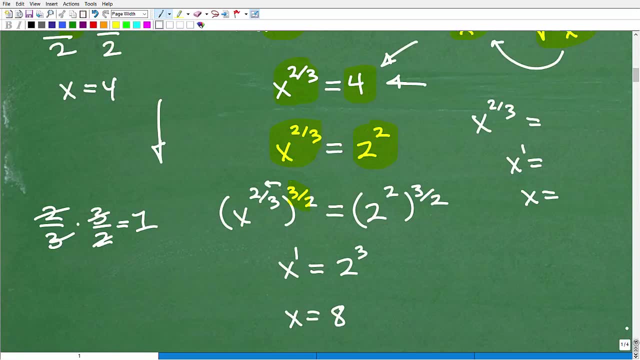 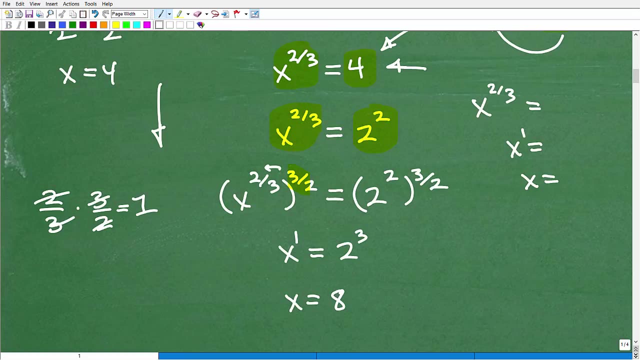 This is going to be one, okay. So I have x to the two-thirds. If I raise that to three-halves power, I'm going to get x to the first power, or x. So that's what I want. But of course, if I raise this side of the equation by three-halves, I have to raise this side of the equation by three-halves as well. 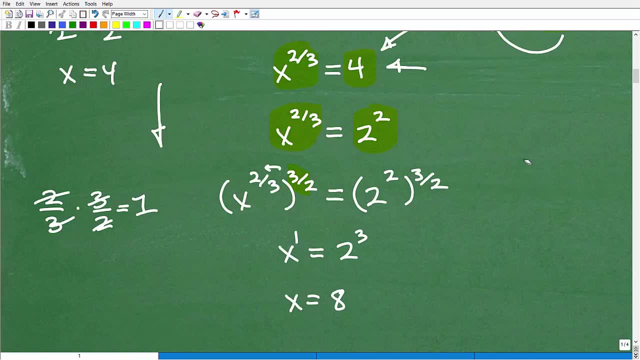 And so now I have to figure out what this is. okay, Let me do this: x squared, x squared to three-halves power, So this is going to be three-halves times two, So two or two over one times three-halves. 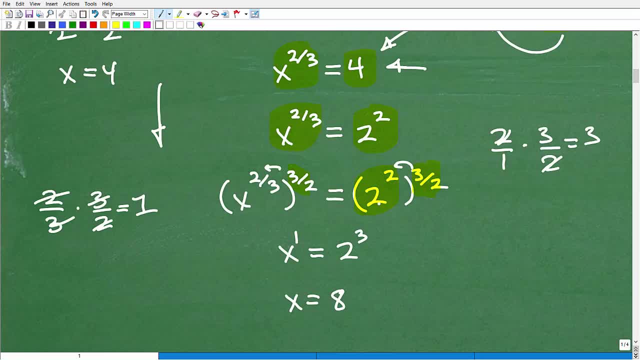 You can see the twos cross cancel and that's going to be equal to three. So two squared, Okay. all this to three-halves power. I'm taking this three-halves and multiplying it by two. It's going to be two to the third power, or eight, okay. 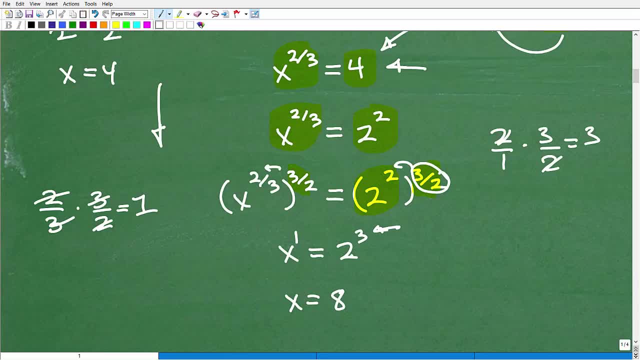 And so now I'm like: oh okay, so x is equal to two-thirds power, And what is two to the third power? Well, that's going to be two times two times two, which of course is eight. 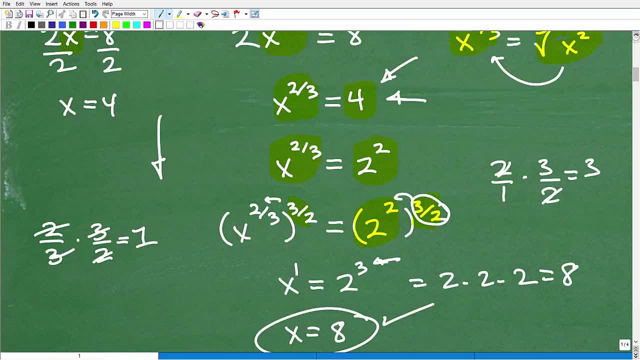 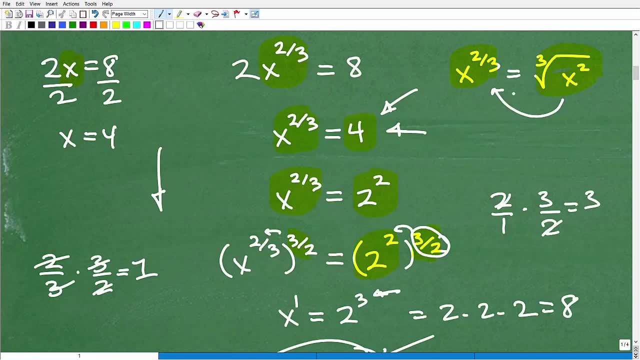 And that is my solution. okay, That is the solution. Now, if we go down here, if we looked at this in this way- meaning if I had the problem here, remember I had x- to the two-thirds is equal to four. 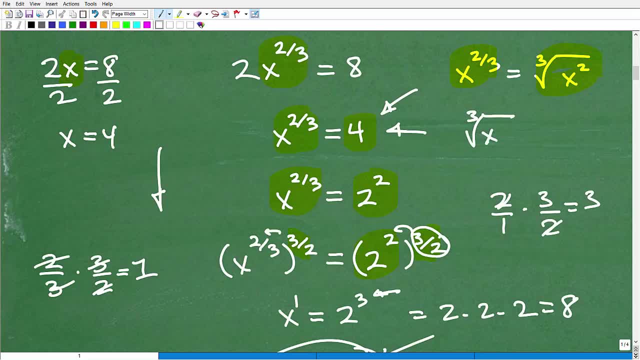 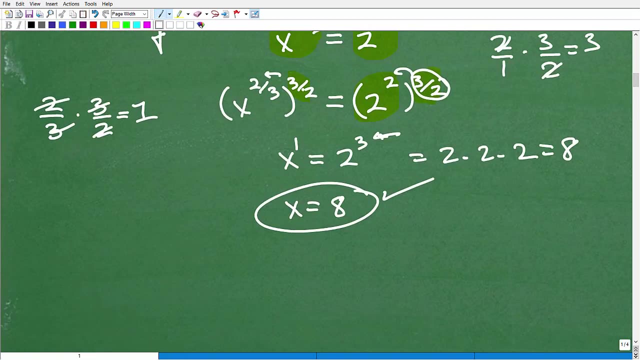 If I wrote it, the cube root of x squared is equal to four. you can see that it would be a little bit more difficult to kind of interpret what's going on. That's what we like to work in rational exponents. okay, Rational expressions are not the same thing as rational exponents. 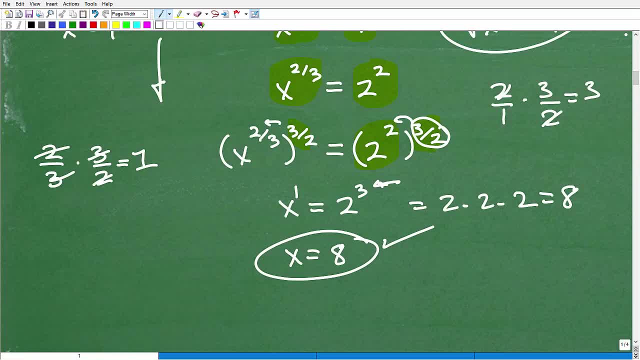 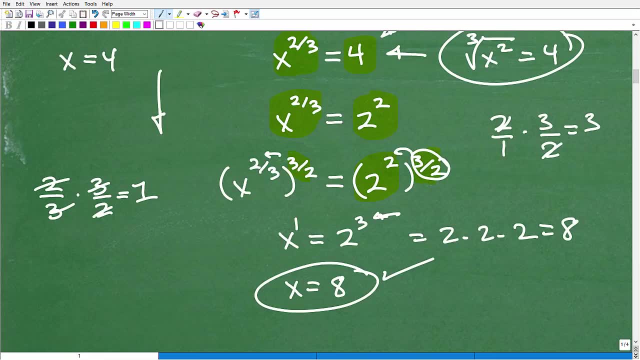 That word rational, though in mathematics means like fractional okay. So this is the best approach, And oftentimes again, you're going to have to solve these equations without the aid of a calculator. But when you do use a calculator, you're still going through the same mechanics. 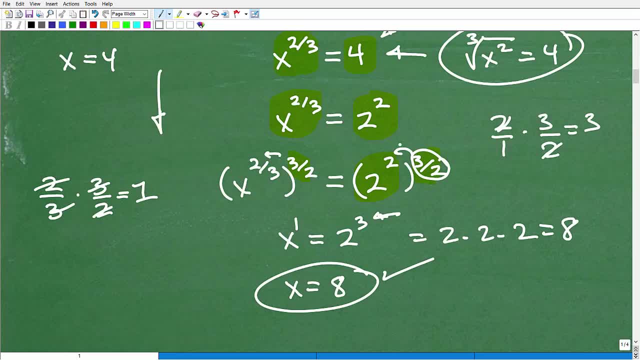 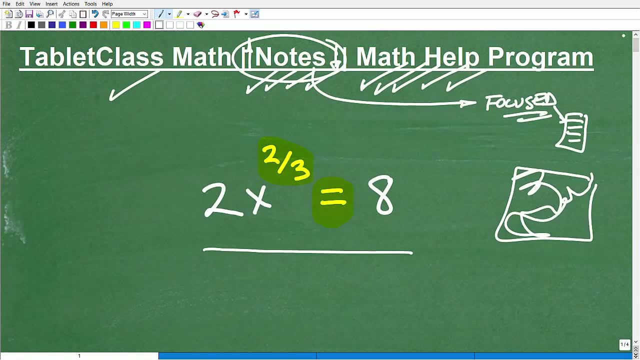 You just won't be able to. you know, oftentimes you know this is not going to work out nicely like this And I've done many other videos on solving equations and you know calculator mistakes- It's a big topic, okay. 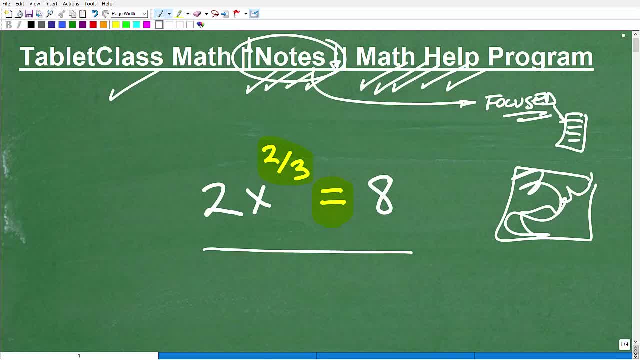 Again, algebra: it builds upon itself. You have to be paying attention, because these skills that you're learning in algebra and mathematics are all interconnected, all interrelated, and they're just not like you know. you learn one thing and then it moves on to the next thing. 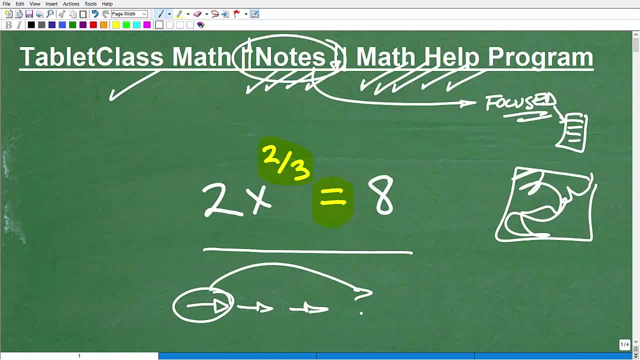 and then you move on to the next thing. The thing that you learn here you may have to learn over here or apply in this particular skill set. It's really cumulative. okay, It's not. you can't like have any shortcuts. you know when you're learning math. 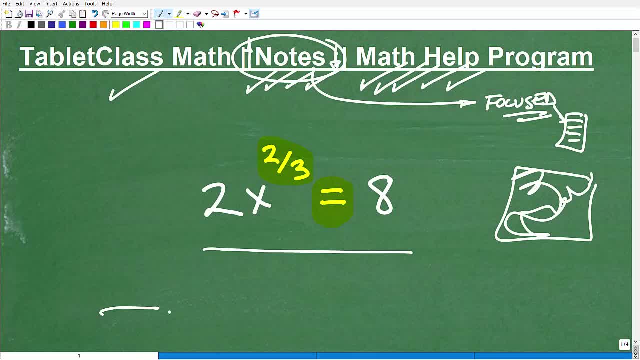 You can't be like: I'll learn. You know I'll learn here, then I'll learn over here, then I'll learn this and this, and then I'll choose to lose. learn this thing over here. That's why it's critical that if you are struggling in math, you get help immediately. all right, 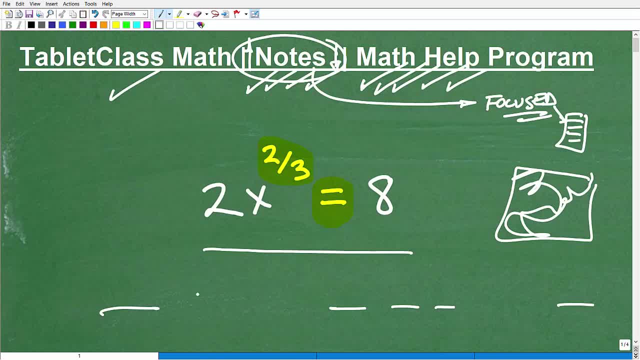 Go to your teacher. That's the first thing you need to do. So if you- or let's say you- failed a particular test, okay, that's a huge thing. If you failed a test, don't be like: okay, I did great in these two or three different tests you know. prior to that. 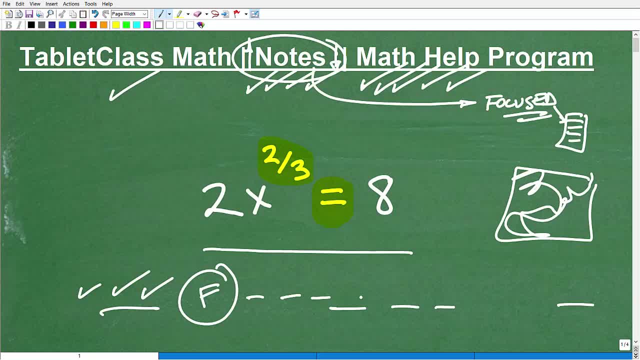 But then I failed this test, so I'll just wait until the next chapter is to come. Do not do that, because that's not going to work out well for you. You need this skill going forward. It may not show up in this next chapter, but it will show up in your future. 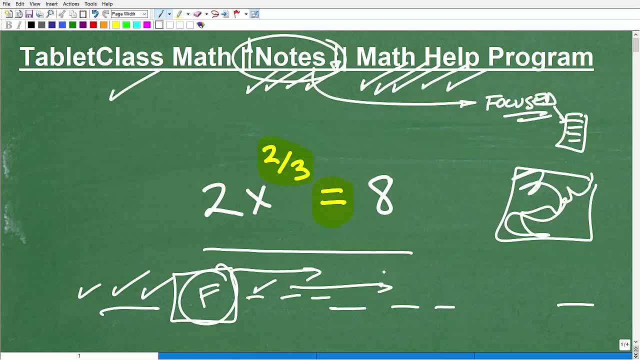 So you have to resolve any misunderstandings And that's why you know the best way to avoid failing okay is taking notes. That and obviously you know learning from a teacher that you like and understand And hopefully you know I could be one of your.